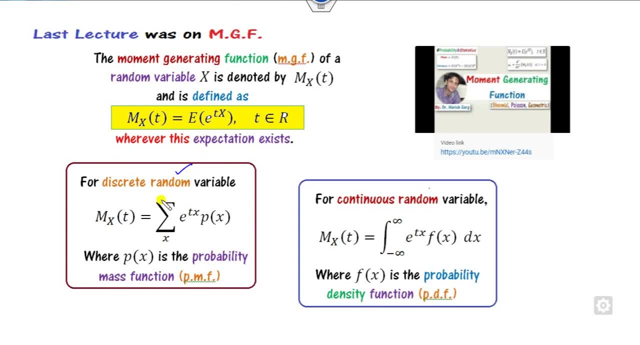 whether it is a discrete or continuous. If it is a discrete random variable, then we can define the expected value as mx, Summation of this, which is a pmf. If it is a continuous, then we can integrate from minus infinity to plus infinity, where f is my pd. We also saw in our last lecture that the moment 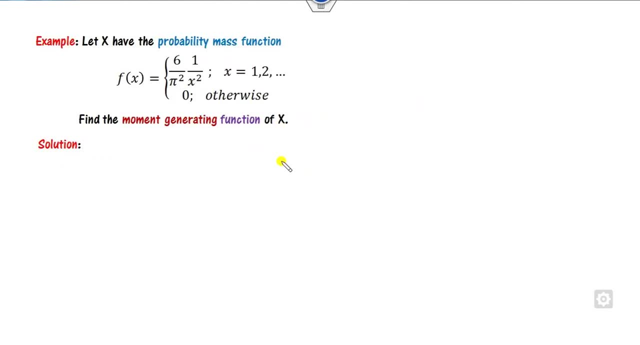 generating functions may or may not exist for all. For example, if you consider the function f of x here and you try to find the moment generating function, which clearly says that the final expression here, which is a divergent series, It means the moment generating function does not exist. 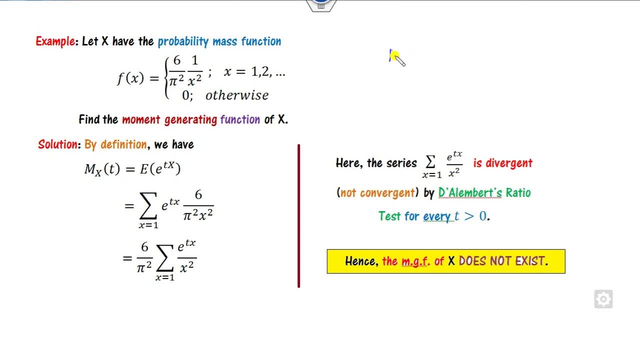 So it means our target is to define a new function which is convergent for all the values of the small t. How you can define that? So you clearly say that this is not defined for greater than 0, but we have to find a function which is convergent for all the t. For that we will need the 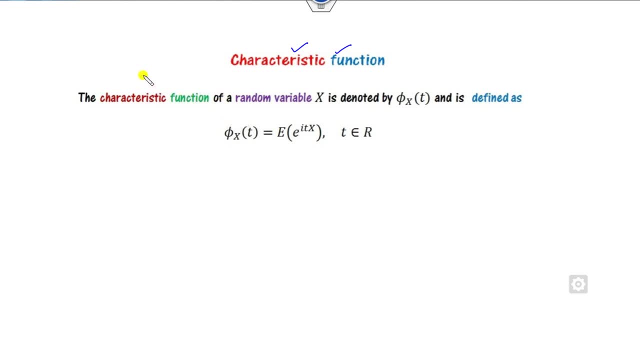 characteristics function. Again, it is a function, so I denoted this as a phi and it is a function from r to r. It is defined like this: It is similar to the mgf, but the only difference here is, in case of the mgf it is my tx, but in case 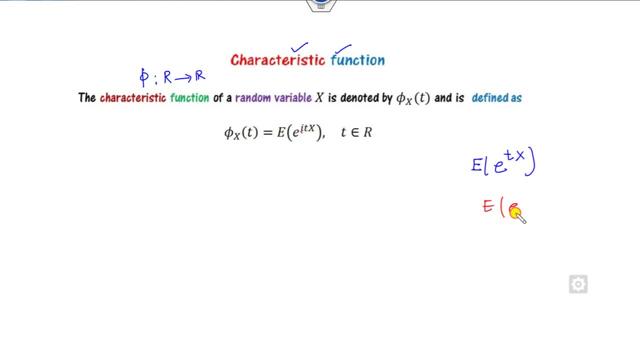 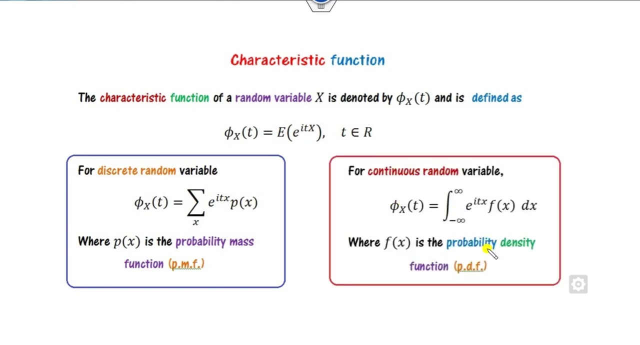 of the characteristics function. it is my e of iota tx. That is the only difference between. here is a complex domain. Again, depending on the nature of the x we can define for the discrete it can be written like here: p is a pmf, If it is a continuous, then we can write as a pd Clearly says that this: 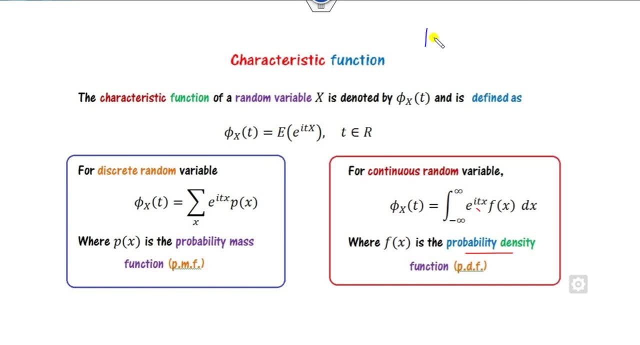 function is existence for all the t, So we can define for the discrete. it can be written like here: how you can say that. So if I take the absolute, because it is a complex number, so we can check about its continuity. So it is my here. this is e raised to power, iota, tx of fx. So what is the? 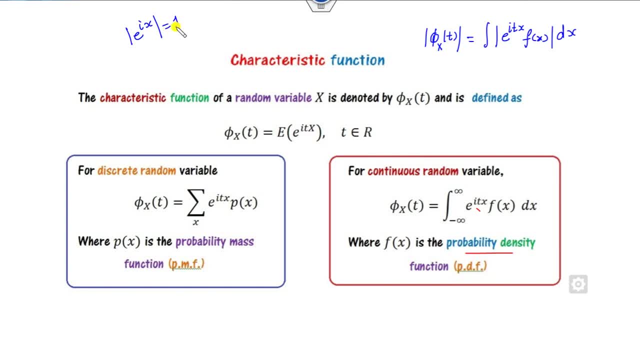 all of you know that e raised to power, iota x. what is the value of this is always 1.. So this value is my 1.. So it is from minus infinity plus infinity. This is my fx dx. So it is always be less than sign, because when you take the modulus value it is always be less than or. 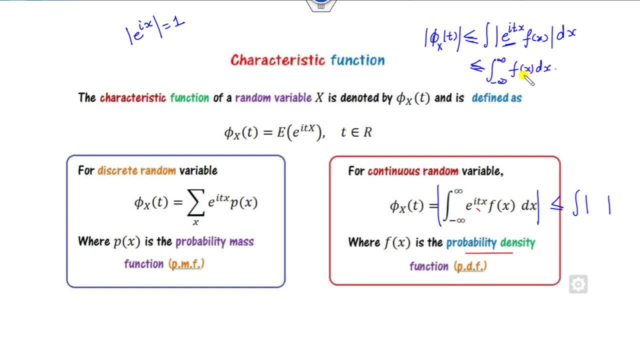 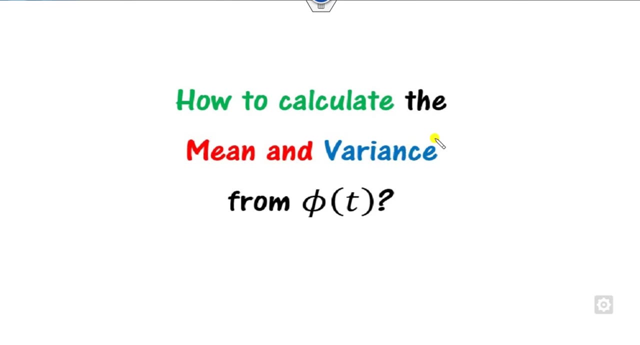 integration of the modulus value. So what is the value of this? because f is my pdf, So this answer is my 1.. So what is the meaning of that? The absolute value is less than equal to 1. That means it is a bound in existence for all value of the t. Now, once you know, once you define the 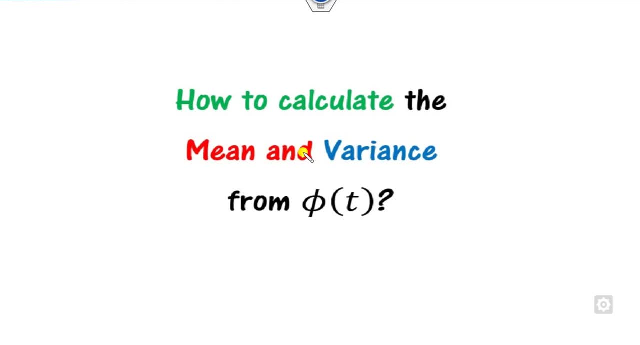 characteristics function, then the major target is how you can define the mean and the variance. We know we can compute. the mean and variance are here, If you look about this expression, and here, similarly, you can define the x Raised to power 3 and so on. So in general, I can define the e, x of r. Clearly says that when x is. 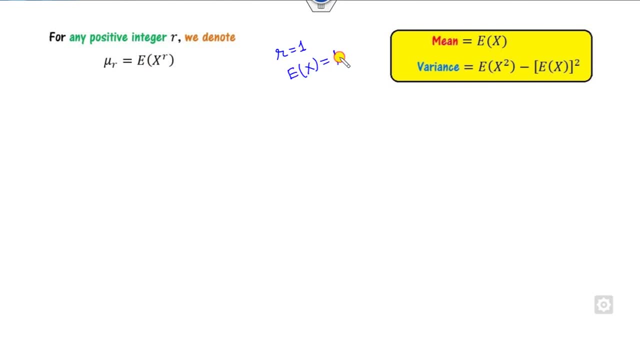 equal to. when r is equal to 1, then it is nothing but my mean mu, 1.. If it is x is equal to 2, then it is the e of x- k. that is a central moment about the origin and so on. Then we can define the two. 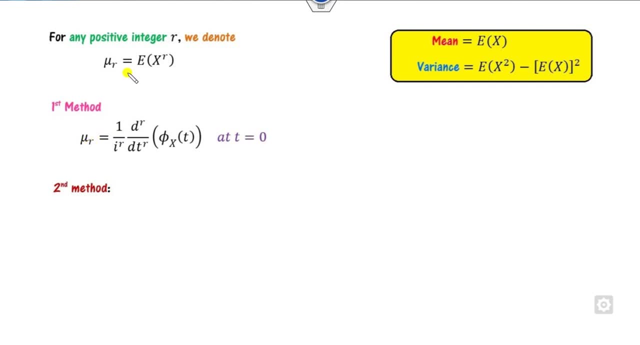 method to compute the mean. The first method is: we can find the value of the mu? r is rth derivative of this. What is the meaning is, If you want to find the mean, what is the meaning of that? It is the first derivative of the characteristics function. Once you know the characteristics, 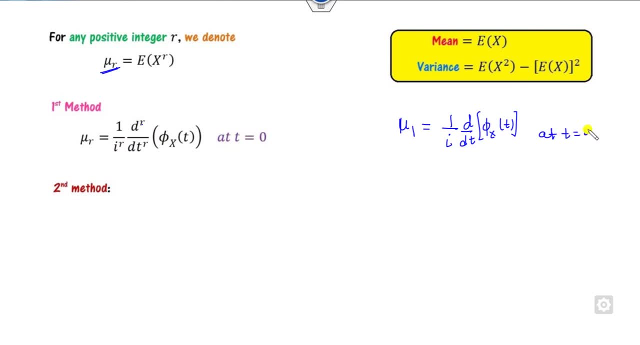 function. we can find the first derivative at t is equal to 0.. Similarly you can find the mu 2.. Mu 2 is nothing but the e of x- k. by using this notation We can define the second derivative at the point: t is equal to 0 of phi x. That is the characteristics function. This is the first. 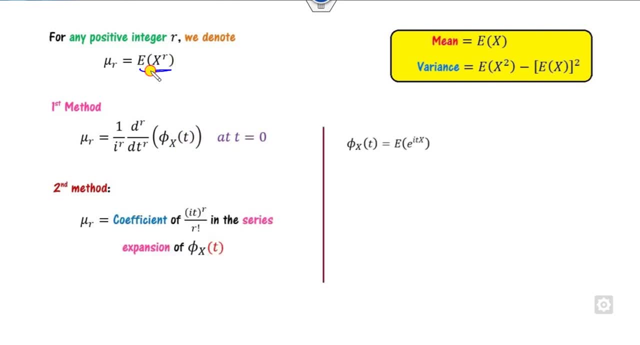 method. Second method is: if we try to open this exponential, If we try to open this characteristics function- this is the e raised to power- We can expand the series if you open them here. Clearly says that. what is the meaning of this? This is my mu 1.. What is that? This is my mu 2, and so on. So 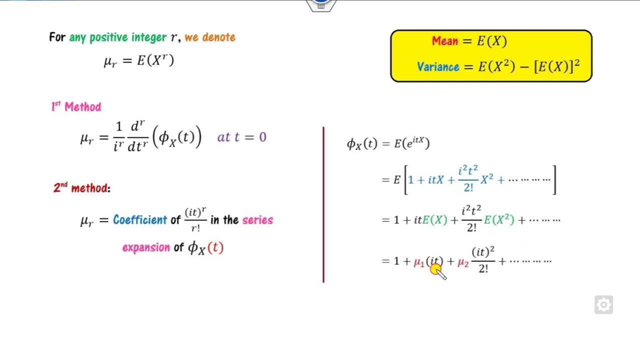 it means we can write like that. So what is that? This is iota t. What is the mu? 1 is That is the coefficient of iota t raised to power r over r. factorial. I can return as 1- factorial, 1.. 2. 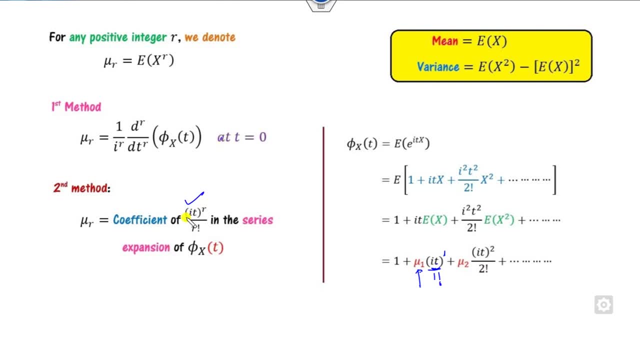 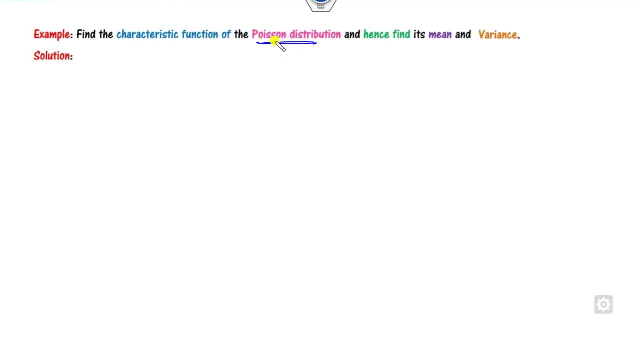 factorial and so on. So this is my here. We will see both the methods. in our next We will see both the examples in the here, For example, how you can define the characteristics, function of the Poisson distribution and then find the mean and variance. Firstly, we all know 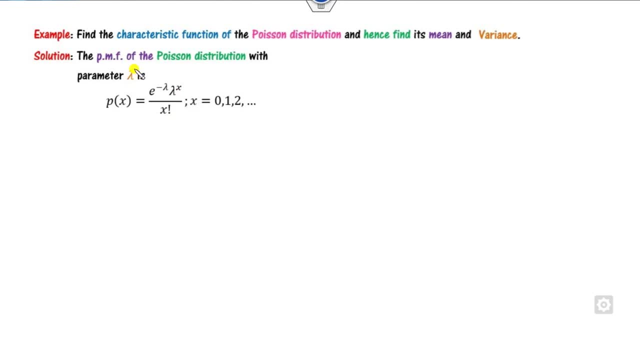 the pmf of the Poisson distribution is my. here The only unknown parameter is lambda and the nature of this lambda is my positive number. Now, by the definition of the characteristics function we can define here, Since it is a discrete function. so we can define like here: 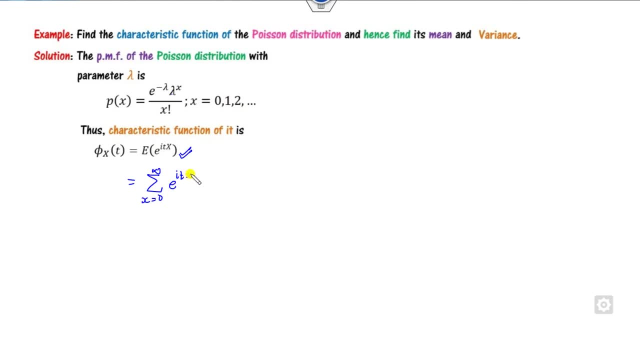 x is 0 to infinity. e raised to power: iota, t, x. This is the definition of this. I can substitute the value of this px at here. This is Now, since this summation is with respect to the x, so it means this part is my constant. I. 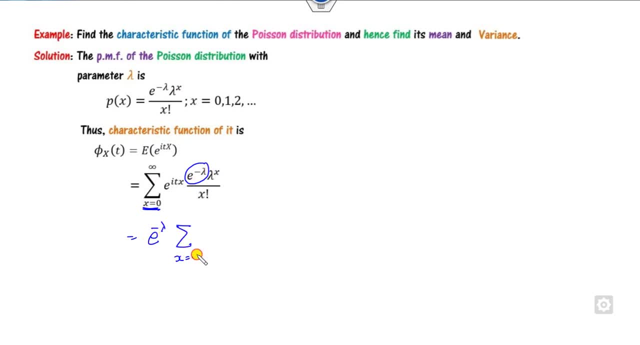 can take this as the outside, and the rest of the part is my here. This: I can take this as power. x is common, So this is lambda of here, So I can write here. So do you know which series is here? Which series will work on this factorial? 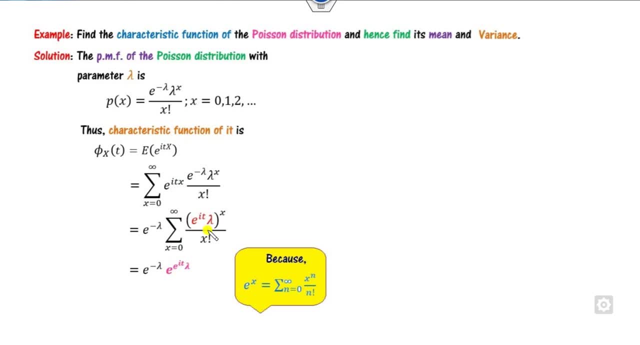 That is nothing but the exponential series. So we can write here as e raised to power of this, because exponential is whatever you have written here, that will be my here. So this is here answer, So we can summarize them. We can take: e raised to power is here, So 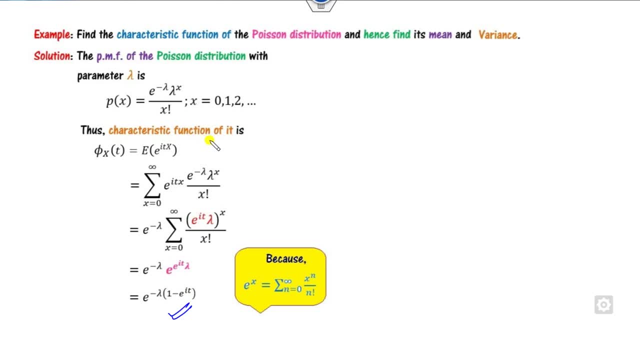 we can write is the characteristics function of Poisson distribution. If you remember that, what is the moment generating function of the here? that is my. this So clearly says that the only difference is replaced instead of the t. it is my iota. Now, based on this characteristics function, how you can define the mean? We know the mean. 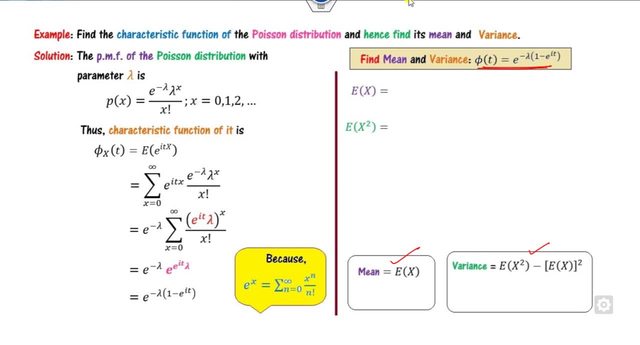 and variances are here. We know this is my characteristics function. So this is my first derivative of this. phi at t is equal to 0. So we can see. So what is the first derivative of this? one by iota is outside. What is the first derivative? e raised to power is same. 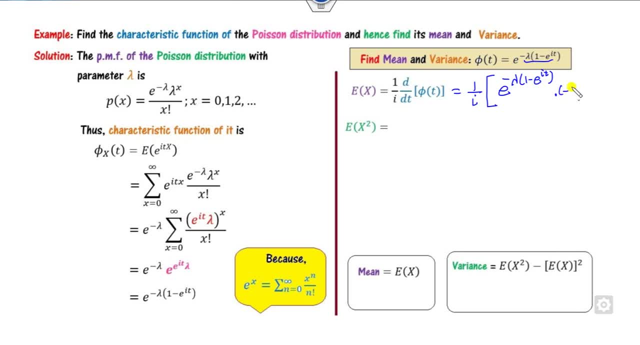 This is my, this one. into the derivative of this. So minus, This is minus, So this is minus of here. and into iota. Fine, This is the derivative of this. How you can find the e of x square. This is the second derivative, So how you can. what is the iota square? Iota. 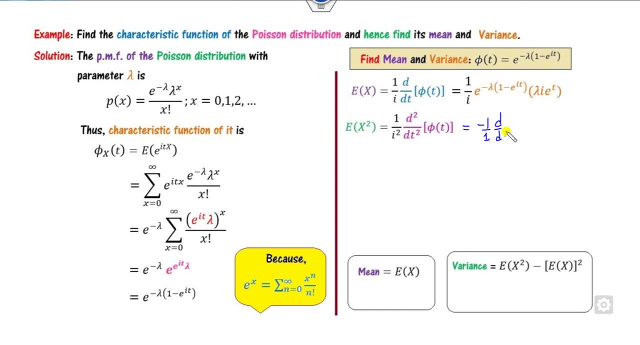 square is nothing but my minus 1.. So what is our first derivative? This is my first derivative, So I can take the first derivative as here. So this minus is because of iota square. Now you can take the derivative. This is with respect to t, So lambda i iota is. 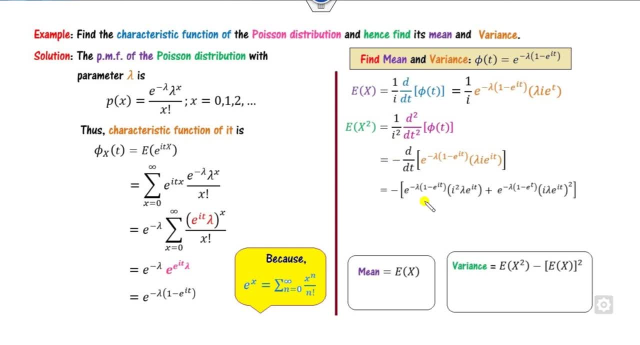 now you can take the product rule. This is my u, This is my v, So I can take like here. Now we have to find all these values: at t is equal to 0. There is no need to simplify that. So what is the value of the e x? at t is equal to 0. This value will be 1.. e raised. 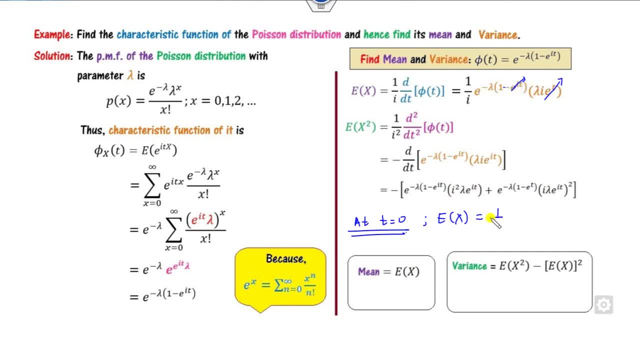 to power: 0 is 1.. So 1 minus 1 is 0.. So this is my 1 over iota. e raised to power 0 lambda i of 1.. So this will be cancelled out. This will be my lambda. 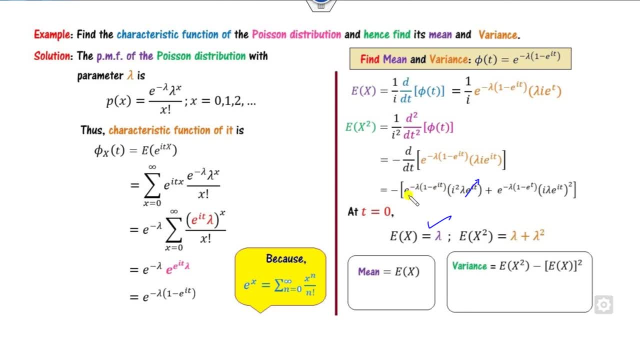 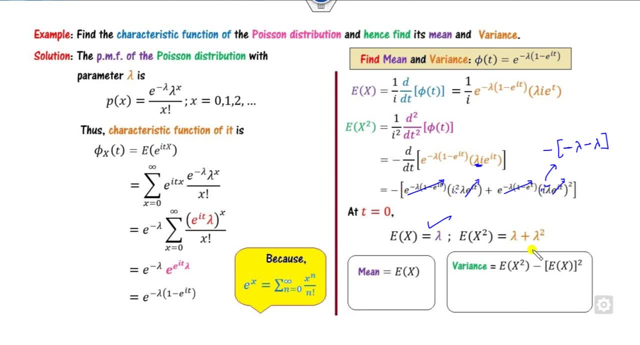 this lambda- sorry, this is a lambda iota. This is iota square, So we can substitute this value here You will get this right answer of here Clearly say that this is 0.. So it is a lambda square, lambda square. That is a minus of this. So you can see, we all know. 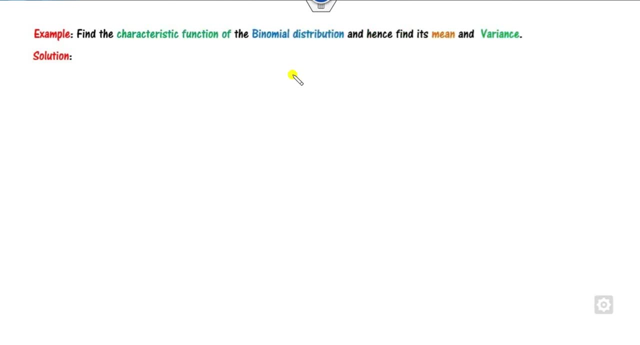 that mean and variance are same. How you can find the characteristic function of the binomial? We all know the MGF of the binomial is my ku plus pe raised to power t of n. So what you conclude? that the characteristic function will be my ku plus pe raised to power iota. 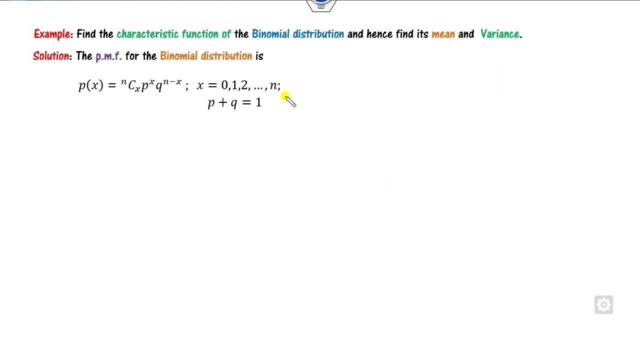 t of n. We will see whether this will be applicable or not. This is the PMF of this. So this is my ku. We can start from here. Take this summation. This is with respect to the x, So we can take. 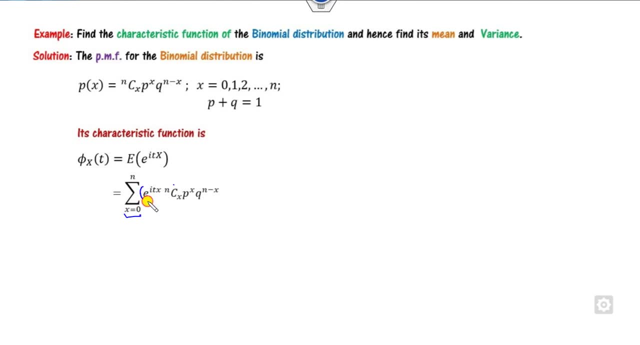 this. everywhere is x is written, We can take the pair of this. We can see, I can take this pair of x. I can return, like here: What is that? This is nothing but the binomial theorem. This is a binomial series. So once it is a binomial series, we can write here. So clearly: 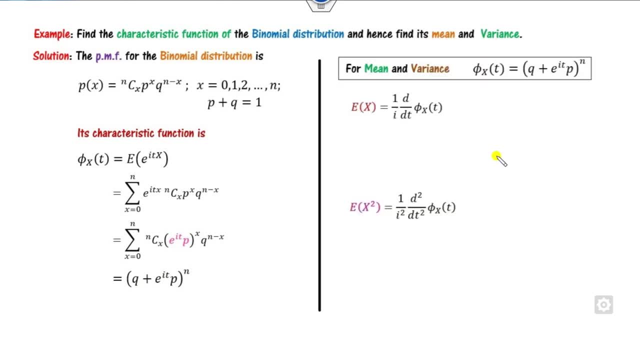 say that this is the characteristic function, How you can define the mean and variance. We can again define like this way: What is the first derivative of here. So we can take: n is outside plus pe. iota t of n minus 1 into ku. is 0 e raised to power. iota t of this into 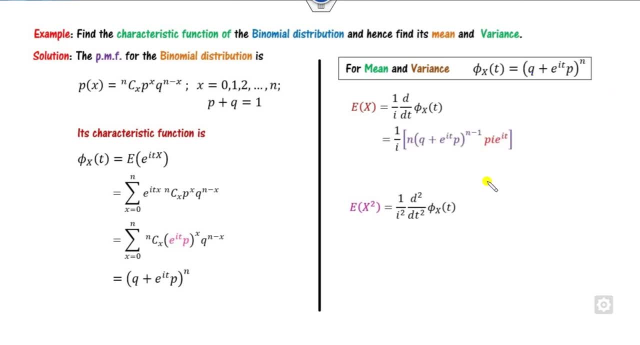 p. This is my first derivative of here. Similarly, you can find the second derivative, or. after that we can simplify it. We will get here because this iota and this iota will be cancelled. How you can find the second derivative? You can find the second derivative of this: This: 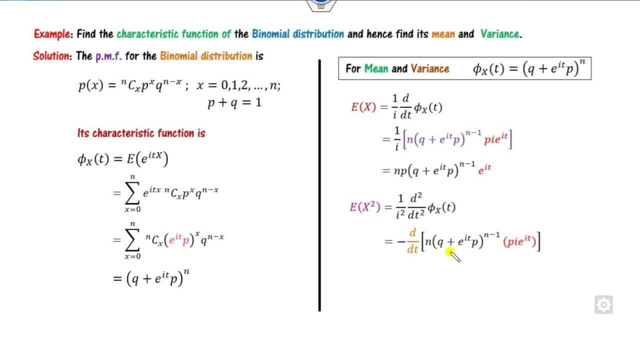 is my first derivative. This minus is here. You can use this. This is a p and p iota is independent of the t. It can be you can write as a outside and then you can use as a product root. We can return here Now. we can take the values at: 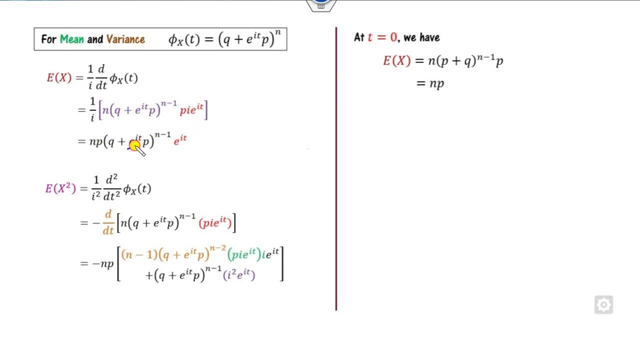 t is equal to 0.. What will happen at t is equal to 0?? This value goes to the 1.. This value goes to the 1.. What is the p plus k in the binomial distribution? This is 1.. So. 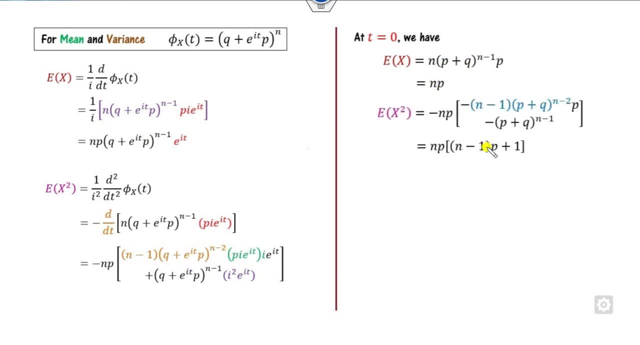 it is n. We can substitute here also. We can see: this value is my 1.. This value is my 1.. This is my 1, and so on. Clearly, p plus k is my 1.. This is 1.. So we can write here So. 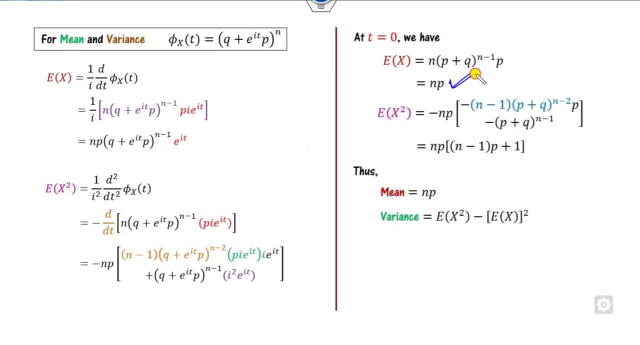 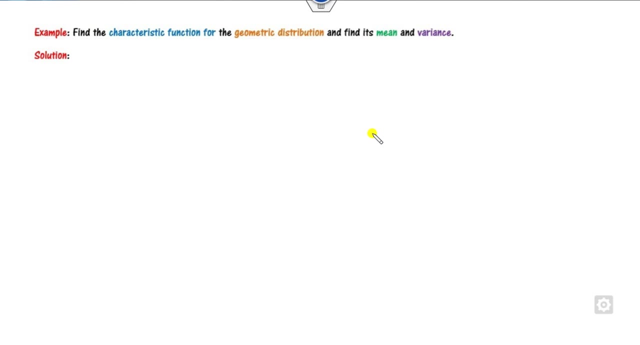 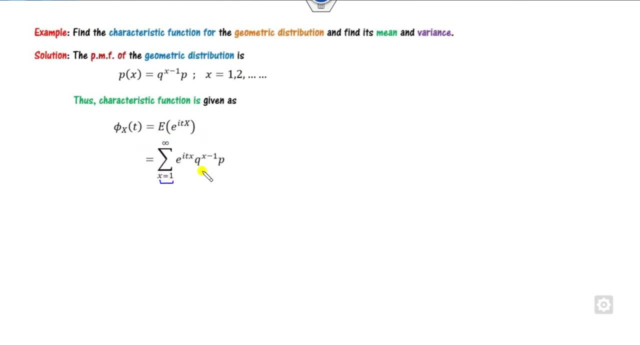 Pmf, So it is n. and these are the geometric distribution characteristics. R crochet, n, x, equipo. This is the geometric concept. Now, what can we call this arithmetic expression? This is the characteristic importance of geometric Hausha representation In your m able, different, complex units. but this is domain By using the definition we can write. 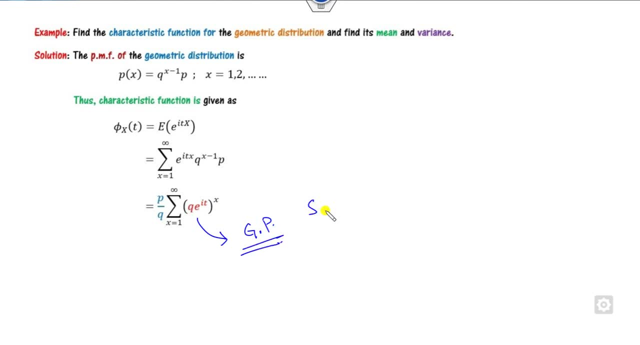 like here, Since this is estimation, start from the 1.. So this p is constant. This ku raised to power peel minus 1.. This is the constant. I can written as 1 to infinity. I can take this part as a commons. so e raised to power iota, t of ku of x. Now do you know which series? 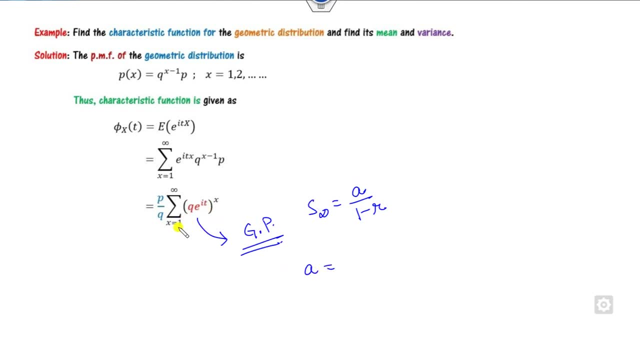 1 minus r. In this case, what is the first term is? The first term is: x is equal to 1.. So this is my first term. What is the common ratio? is The ratio will be my again here, So I can substitute. 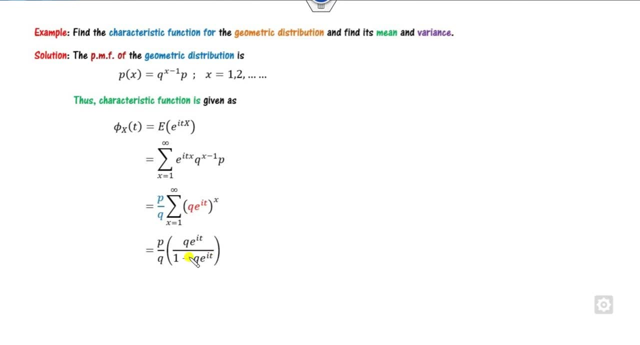 these two values here, We will get this one. So Kalilji says that this q and q will be cancelled out. We can write as a characteristic function How you can find the mean and variance. We all knows the mean of the geometric distribution is 1 by p and the variance will be my ko by p. 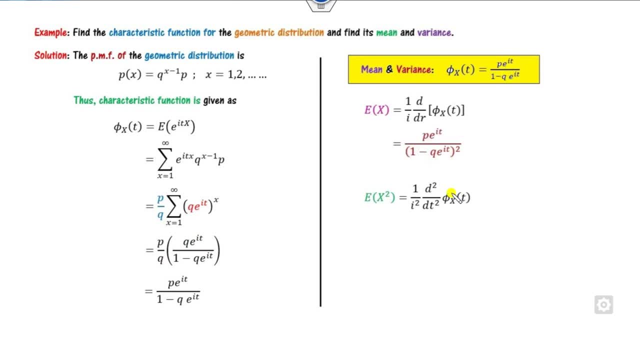 square. So we can take the first derivative of this. We can write here: After the first derivative, you will get this expression. You can find the second. This is a minus 1 and you can find the first derivative and then you can find the second derivative. You will get this as the expression. 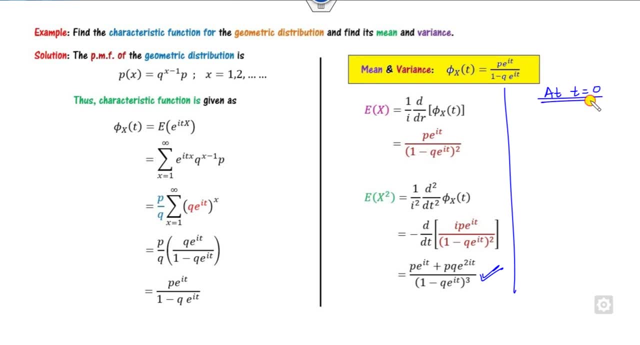 Now again you have to check at. t is equal to 0.. What is the value of the ex? You can substitute: x is 0 here. this is my 1, so it is p. this is 1 minus q is a p. it's a p square. it is my 1 by p. 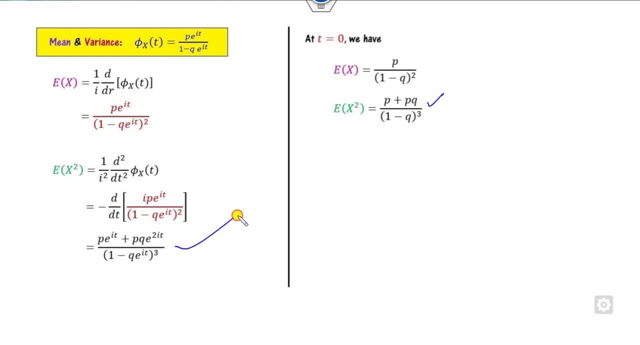 similarly you can substitute here. you will get this expression here. so therefore you can simplify it. this is 1 by p. you can simplify it. p is a common 1 plus q. this is my p cube. so if one cancel out it is 1 plus q upon p square. therefore, variance is my, q upon p square, and mean is my. 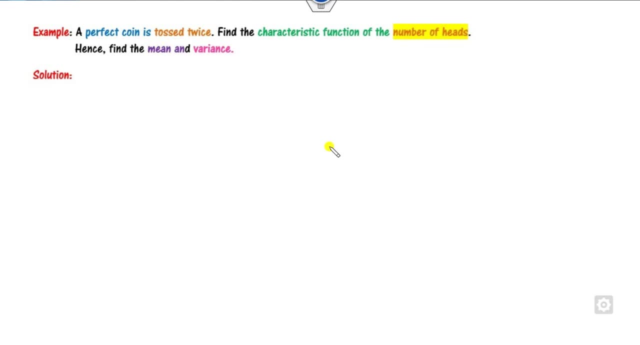 here. okay, look at these some examples. so a perfect coin is tossed twice. so a coin is tossed twice. okay, find the characteristics function of the number of the heads. so there are the two methods. the first method: i will tell you a very simple: if the coin is tossed two times, 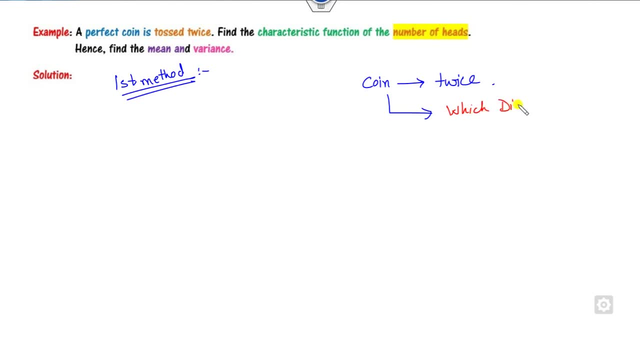 which distribution will be here. can you find the? which distribution is there? yes, this is a binomial distribution. once it's a binomial distribution, how many times you toss the coin? two: what is a p? what is that? this is a head. so what is the probability of getting the head on the one? 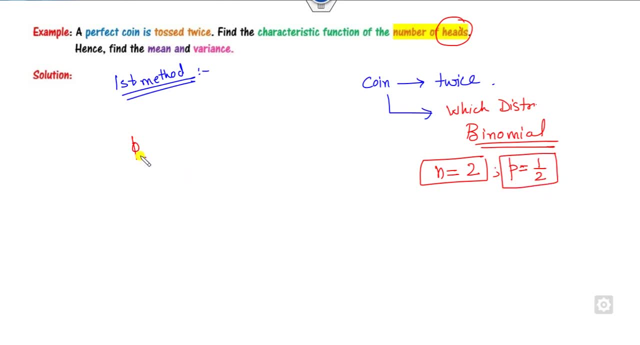 tossing the coin. this is here. and what is the characteristics function of the binomial distribution? this is q plus p, e raised to power iota t of n. this is the binomial poison you characteristic function. Now you can substitute it to the value: q is half, p is half of n is my. 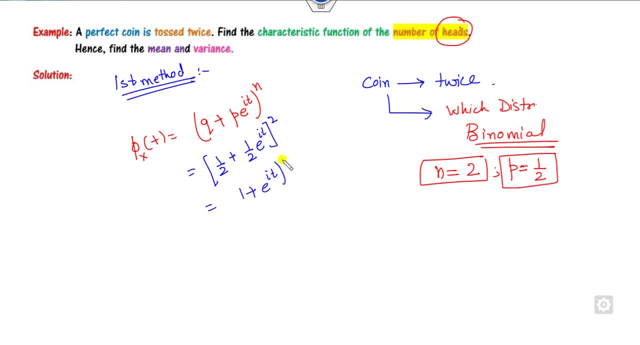 2. So I can return as: iota t square divided by 4 is the right answer. Now, once you know this is a binomial distribution, what will be the mean of the binomial distribution? Mean is my np. So 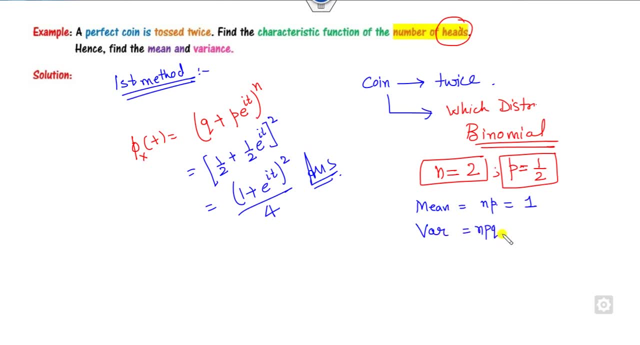 that is a 1.. What is the variance? is npq. So that is a half is the right answer of this problem. This is the first method. This is the second method. If you do not remember the characteristics function of this binomial distribution, then how you can do that. We can try to write the. 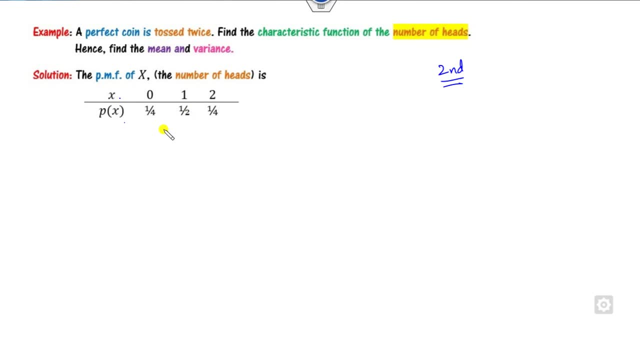 random variable and the corresponding probability. These are the two cases. Now we can apply the binary definition. Now here, what is our domain is? x is my 0 to 2.. So when x is 0, so e of 0, p 0 plus when x is 1, this is my p 1 plus. 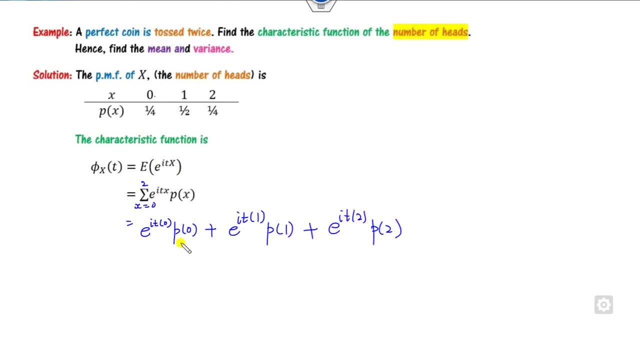 x is 0 to 2.. It is my p 2.. So we can substitute the value of the p 0 as 1 by 4, p 1 as 1 by 2 and p 2 as 1 by 4.. So e raised to power 0 is 1.. It is 1 by 4.. It is half e raised to power t plus. 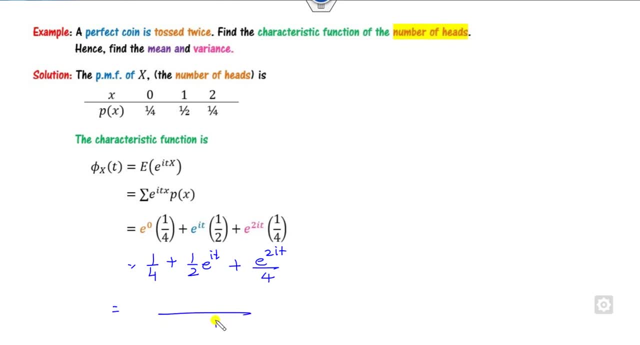 e raised to power, iota t by 4.. Or you can take 4 as the LCM and you can see this is my expression, which can be written as of e raised to power by 4, which is same as that of the first method. How you define the mean and variance? Again by using the derivative of this. 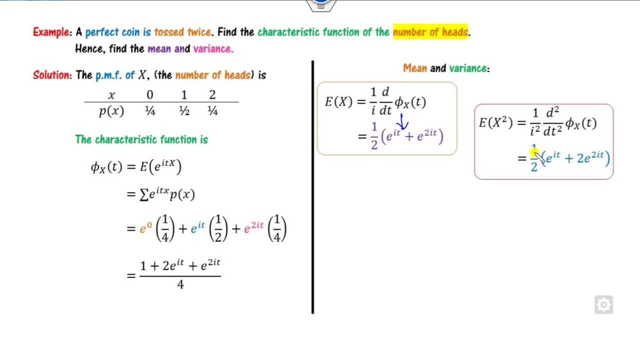 you can take the first derivative, you will get as here. If you take the second derivative, you will get this. Now you can find the values: at t is equal to 0. So what is the value of the here? At t is equal to 0,. this is my 1 plus 1.. So answer is 1.. At t is equal to 0, what is the? 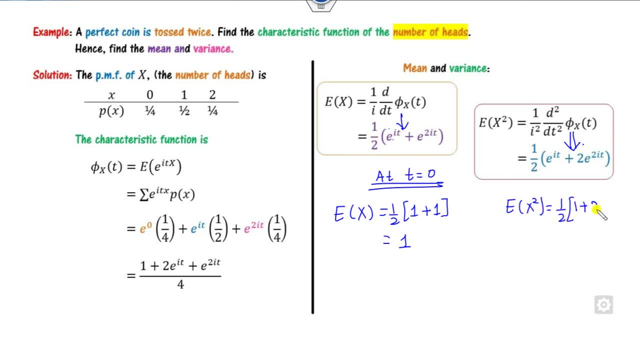 value of the e x square. This is half 1 plus 2.. That is my 3 by 2.. So therefore, mean is my 1.. This is my mean. Variance is e x square minus e x whole square. That is my 1 square. It is the right Look about this one. So in this case, 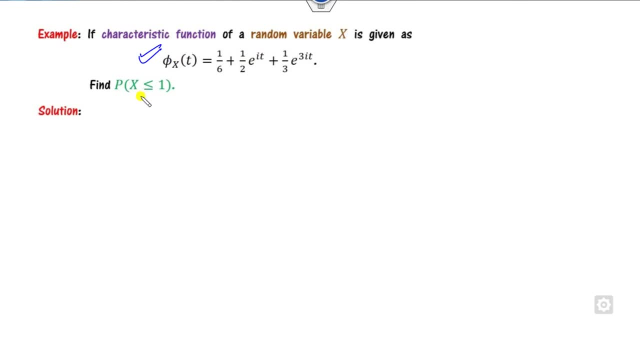 characteristics function is given to you and you have to find the probability of this. So look at that If you are trying to find the mean, if you are trying to find the variance, but you have to find the probability of this. So look at that If you are trying to find the mean. 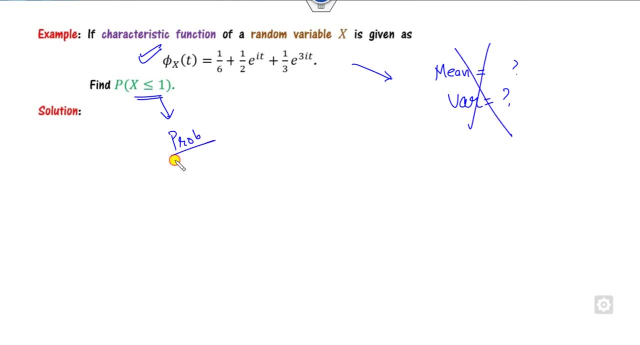 if you are trying to find the probability. there is no need of this. You have to find the probability. So, first of all, this is the plus sign. What is the meaning of that? This problem is my discrete random variable. Once it is a discrete random variable, you have to draw this. 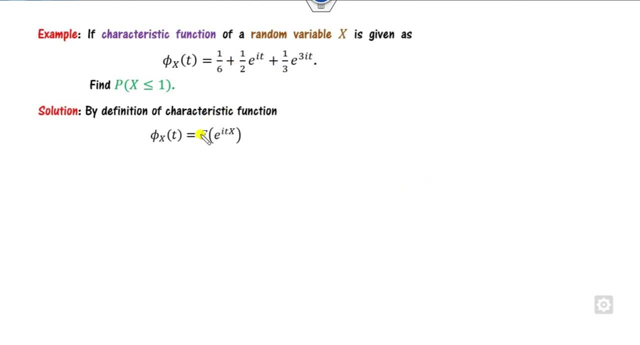 table. So what is that? I can express each of the quantity with the help of characteristics function. We can start from here Now. if you open this, you can write like this way, because x start from the 0 to up to. 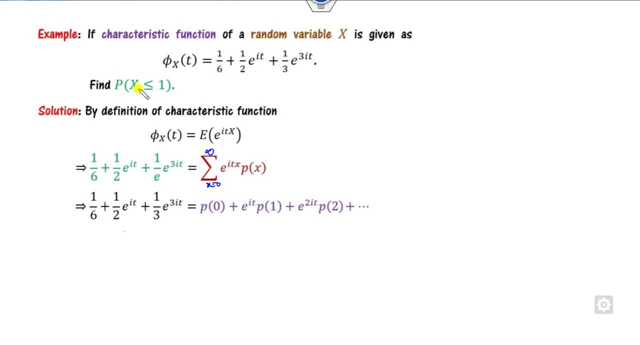 How many there There are. infinity, because nothing is given to you about the variable x. We can write like here: When x is 0, this is 1 and so on. Now, if you compare them, this is a independent of exponential part. So it means p of 0 is my 1 by 6.. Coefficient of e raised to power t. 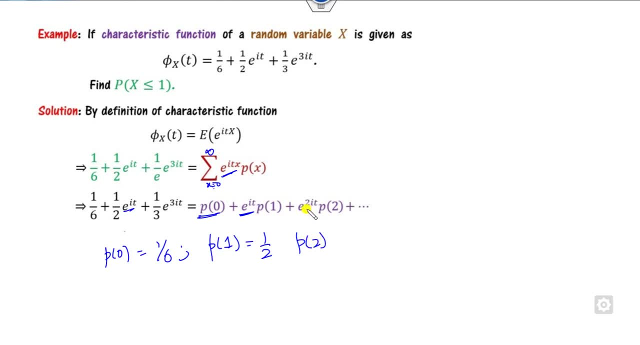 this is my 1 by 2.. What is the p2 is Coefficient of e raised to power 2.. There is no term of there. This is 0.. This part is coefficient of 3 raised to power. This is my p3, because you can see there is a next term is my here plus so on and the rest all the. 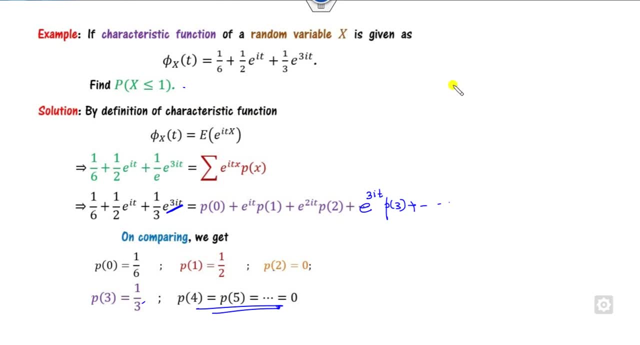 parts are my 0.. Once you are identify this, then how you can write this value of this Less than equal to 1.. That means x is equal to 0 plus x is equal to 1.. So you can write this value as what. 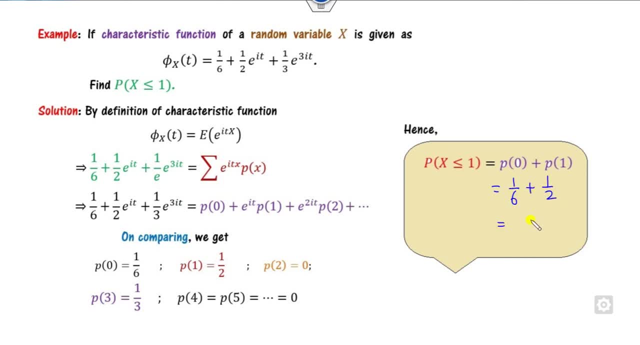 is the p0?. 1 by 6,, 1 by 2 is the right answer, or you can say it is a 2 by 3.. Otherwise you can write like this table: You can see that values are 0,, 1,, 2 and 3.. So what is the value of the 0 is 1 by 6.. This is my 1 by 2, 0 and this. 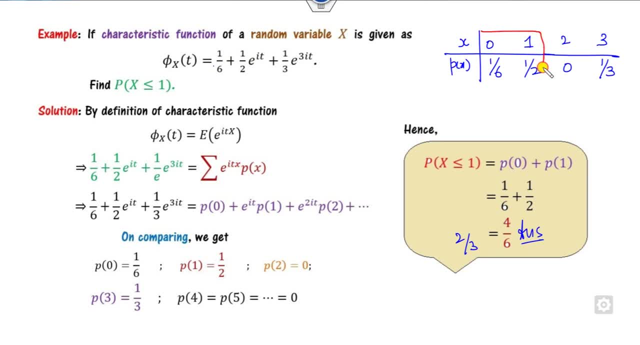 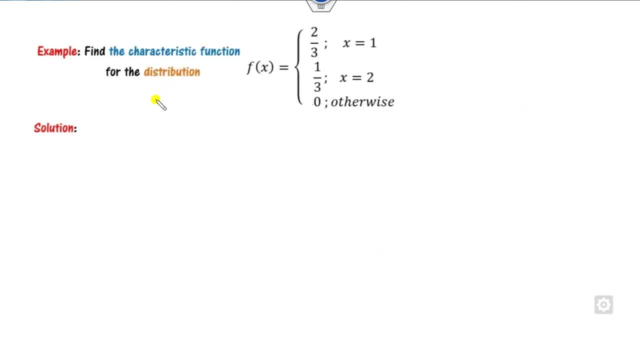 is my 1.. Rest, all are my 0 and your target is to find this answer, as here, which is same as that of this. Okay, look about the another one. Find the characteristics function of this. So clearly say that these are the single point. So it means these are my discrete distribution. Once they. 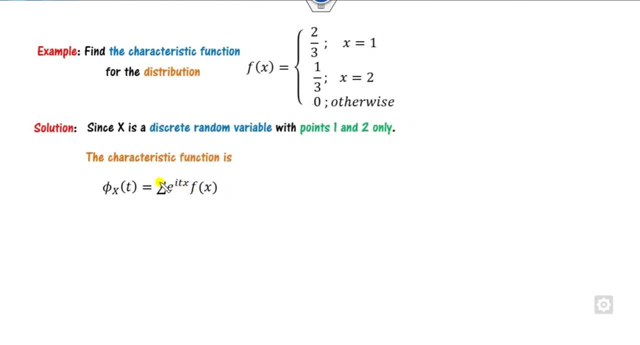 are discrete distributions so we can write like here. That is why there is summation sign. So now this value is my either 1 or 2.. So if I start from the 1, e raised to power iota, t of 1, f of 1 is my 2 by 3 and f of 2 is my 1 by 3.. That is you can take as.